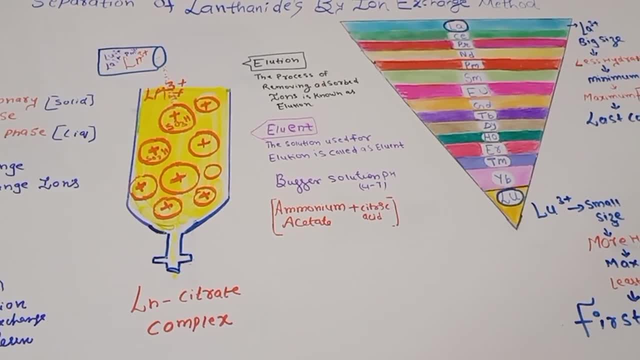 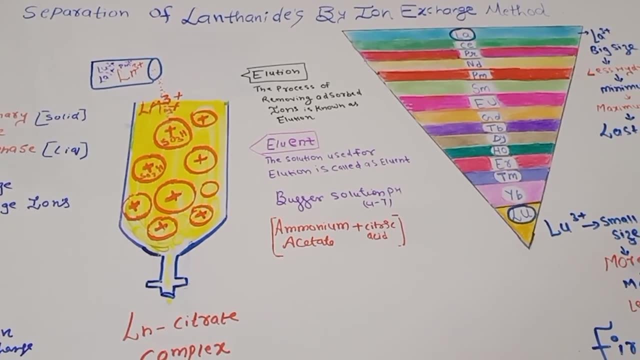 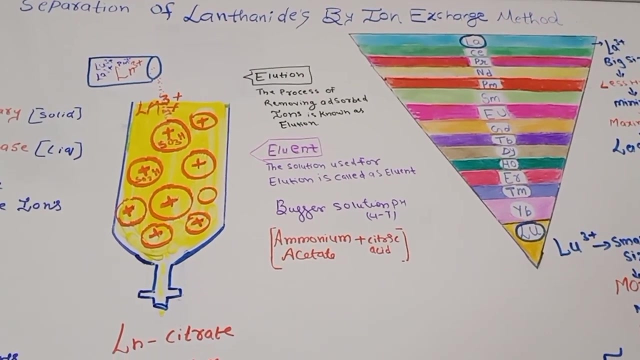 uploaded of this chapter. Now, this question is very important exam point of view, So just let us understand this topic. Okay, so what are the our ion exchange method? If you have know, if you have previously know about the chromatography, so it is a type of a chromatography. 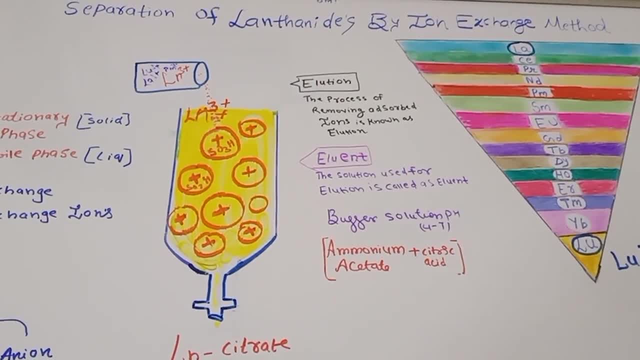 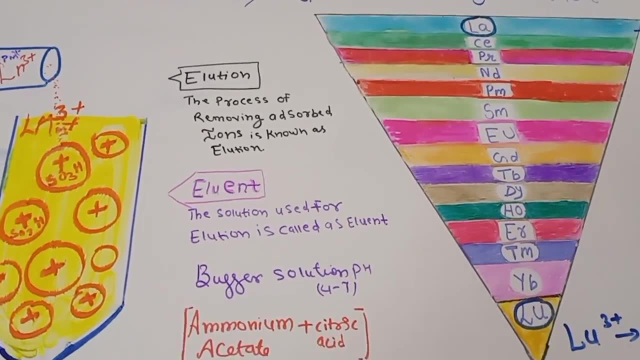 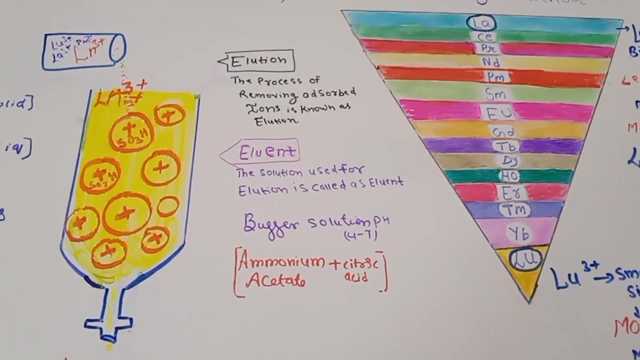 means in this type of ion exchange method we are going to exchange our lanthanide On the basis of their ionic size. as we all know, whatever lanthanide series, it starts from lanthanum to lutetium. So in the ion exchange method, according to the size of 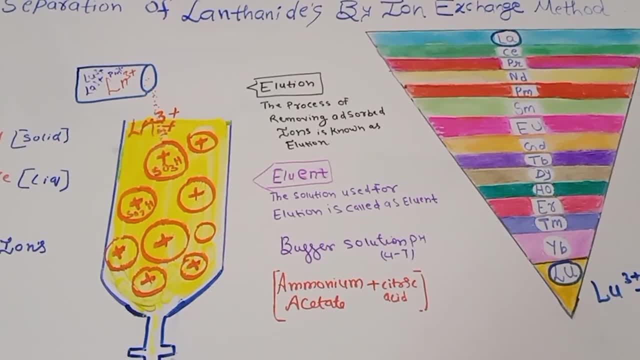 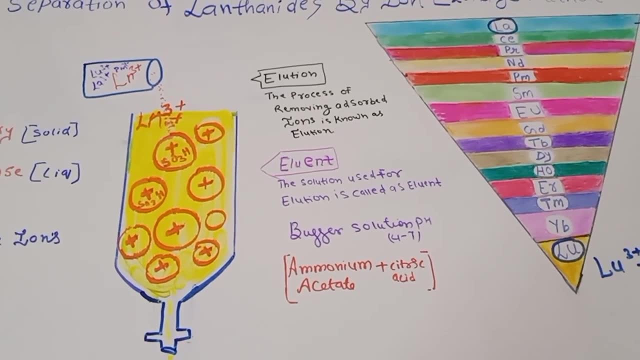 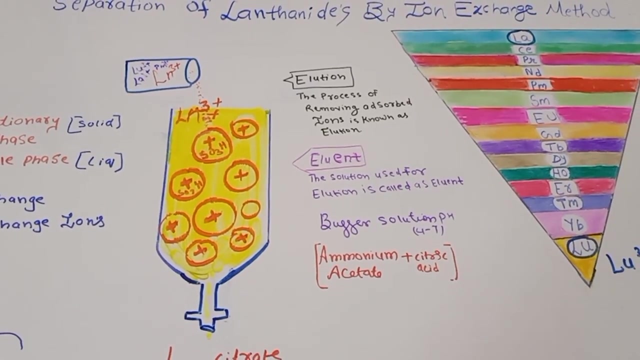 the lanthanides. we are going to separate the lanthanides as we can say that there is a as due to the lanthanide contraction, the size where is very small. So it's very tough to separate the lanthanides by the normal method. So the ion exchange method is used for the separation of the 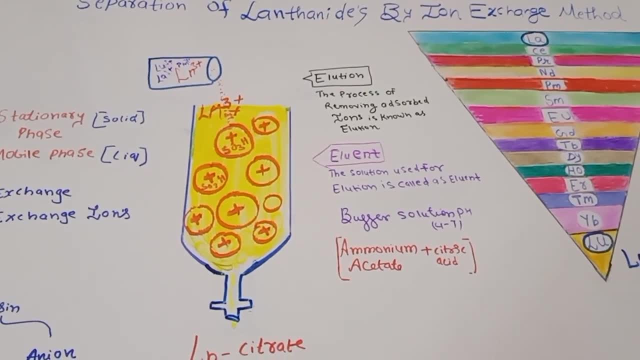 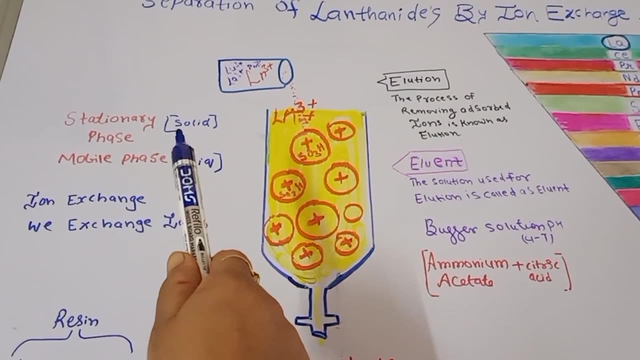 lanthanides. So let me explain you first the basic terms which we will use here. For example, in any chromatography there is one stationary phase, So we can take any stationary phase as a solid and one is mobile phase. And what we are going to do in this method, we are going to 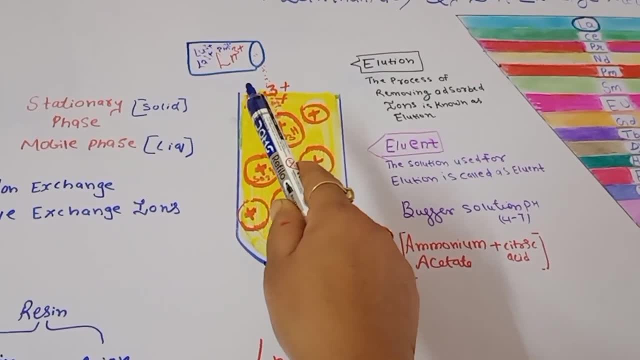 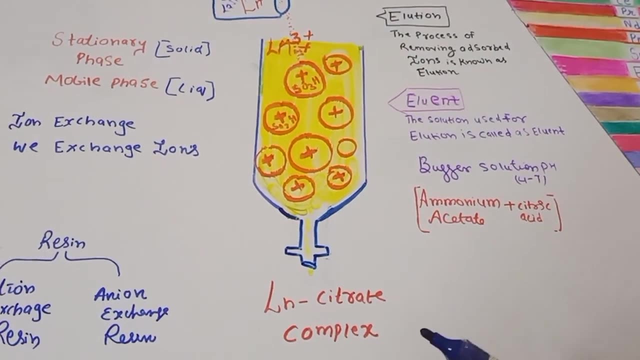 exchange the ions. as we know, the common oxidation states of the lanthanide is plus three, So all the lanthanides ions is in the form of ln3 plus. we have written here. So first, what we will do, we will take a mixture of our lanthanides. 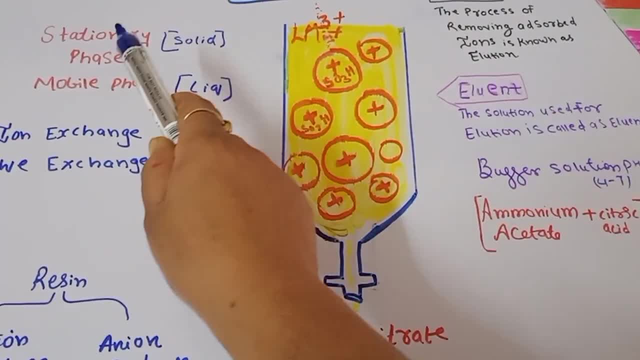 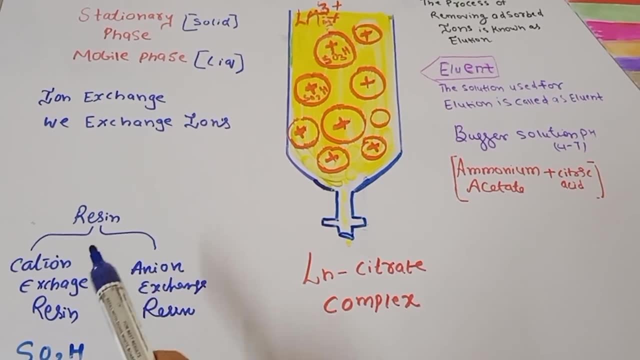 And we will prepare one stationary phase. So in this stationary phase, what solid we are using to prepare this stationary phase? we will use the resins. So resins can be of two types, that is, the cation exchange resin or the anion exchange resin, As the lanthanides are having. 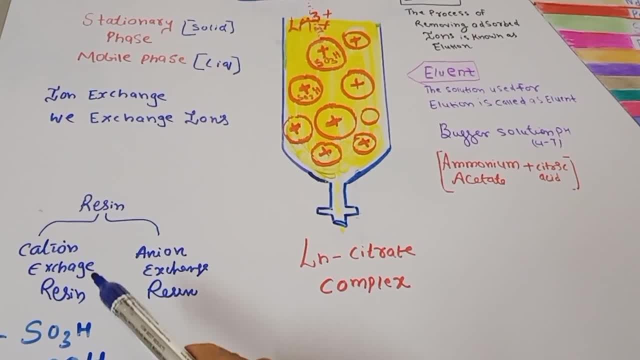 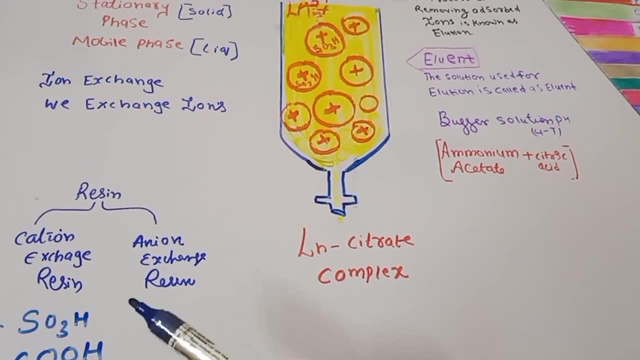 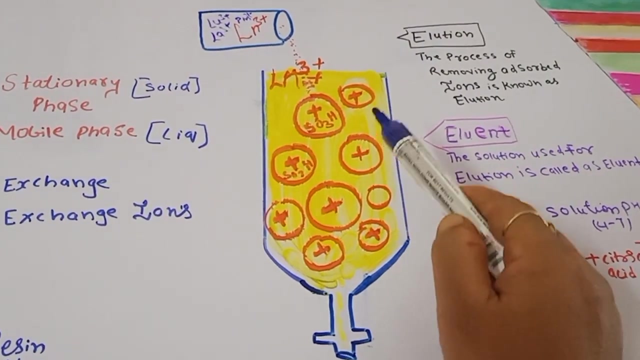 three plus charge means they are the cations. So we will take our cation exchange resins here, for example SO3H resins or the carboxylic group acids resins. So what we will do, we will first separate the cation exchange resins with the help of our stationary phase. all these solids. 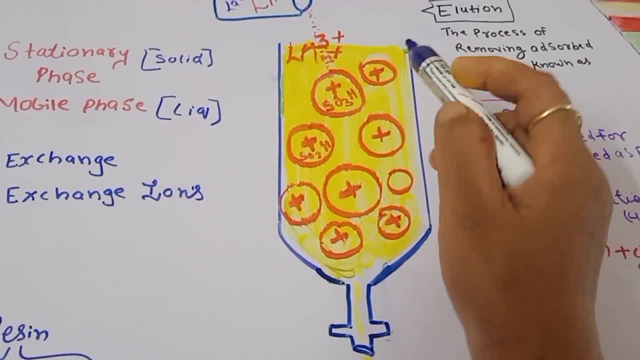 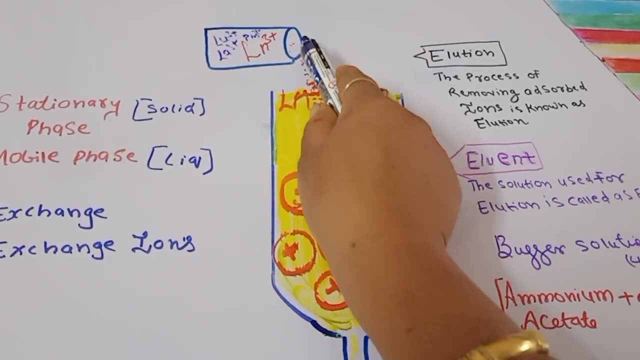 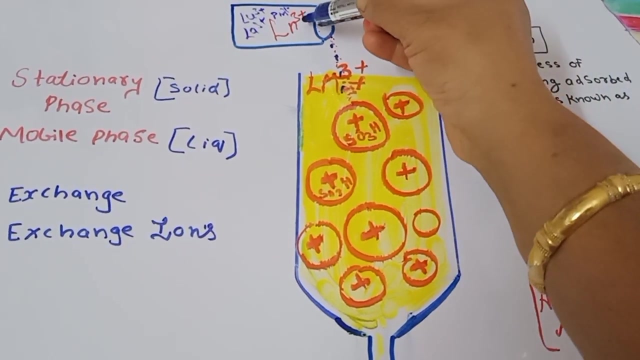 So here with the red circles I have just made the resins and you can see SO3H. So what happens when we take the solution of the lanthanides in this weaker? we will just show the solutions of the lanthanides which we want to separate. What will we do when we will flow this mixture of the? 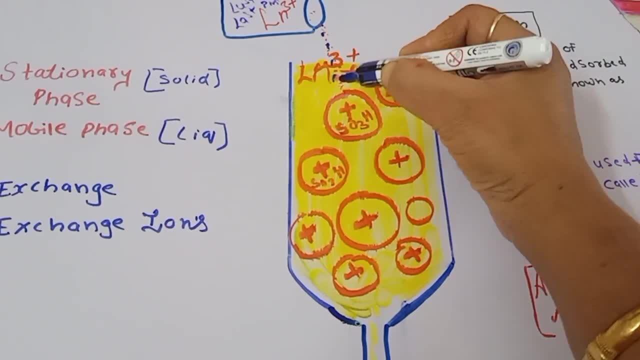 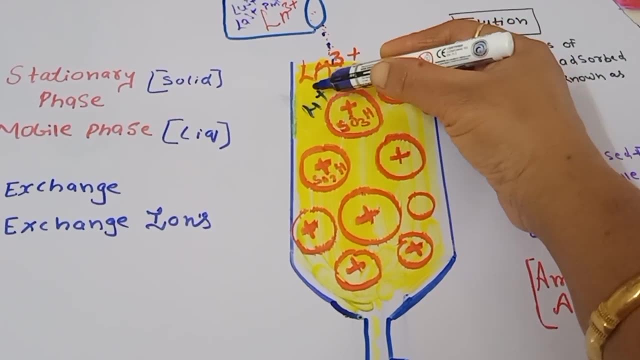 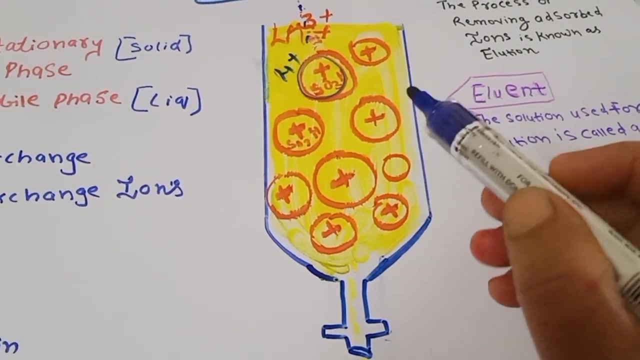 lanthanide three plus. So it will exchange. you see this SO3H is here, Naah, Naah, Naah. what will be there? this, our ln 3 plus will get exchanged with h plus and it will get attached with the resins. means what happens when our any resins- means cationic resins- are there in the 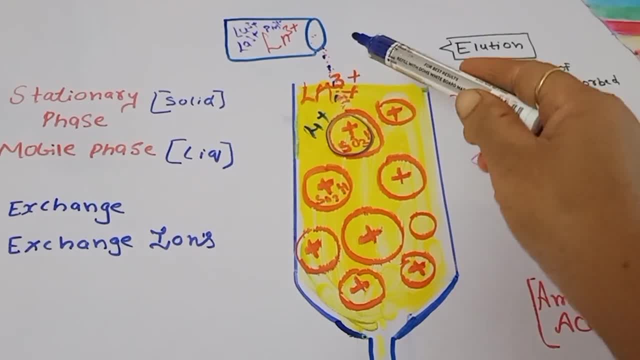 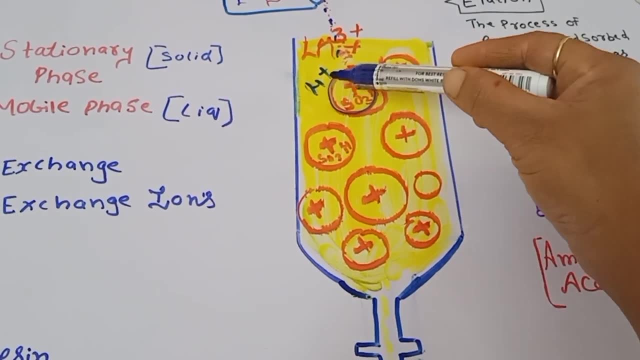 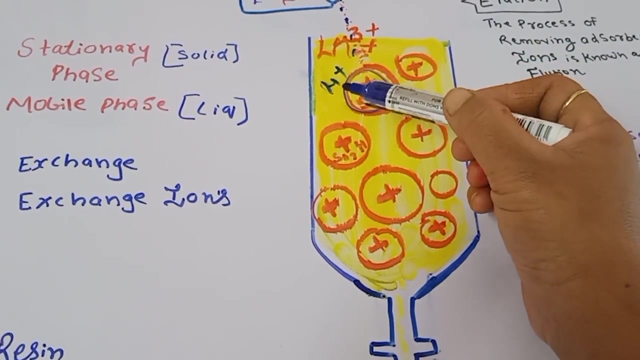 stationary phase. so what happens when we flow the solution of our lanthanides? all the lanthanides will come and they will get contact in with the resins and they will exchange the cation. so this is a type of a cation. exchange means our ln 3 plus will exchange with h plus and ln 3 plus means 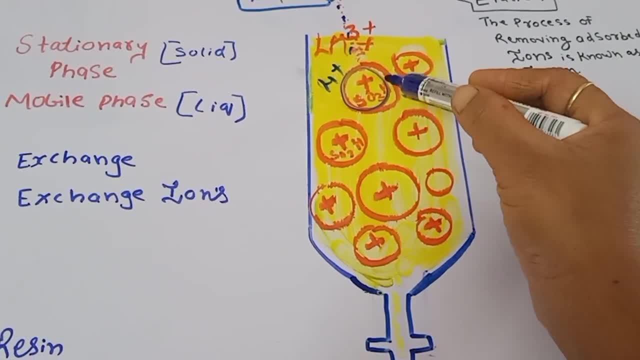 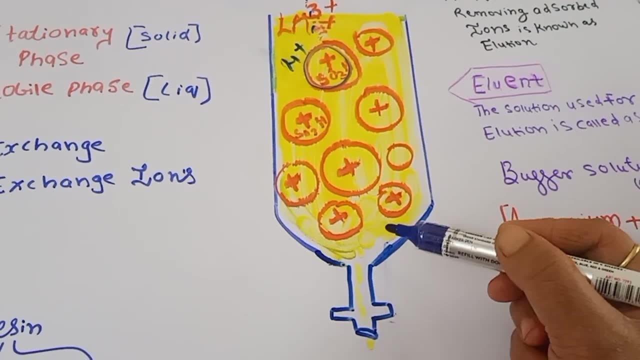 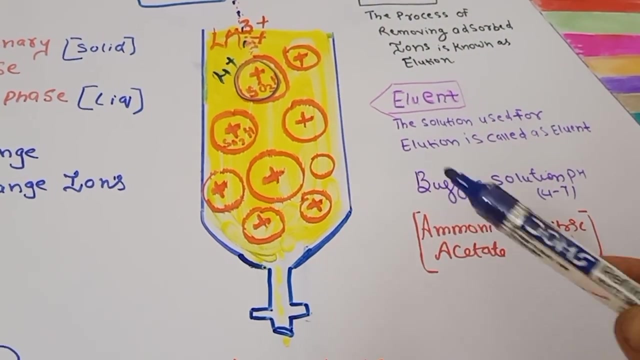 any lanthanides will attach with our SO3H molecules in place of h plus. so, one by one, all the our lanthanides will attach with the resins. and in last, what we have to do, we have to then separate this from. this column means so how we will separate. so for the separation we will use, 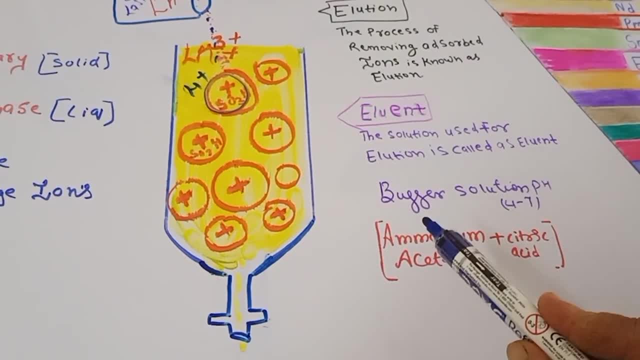 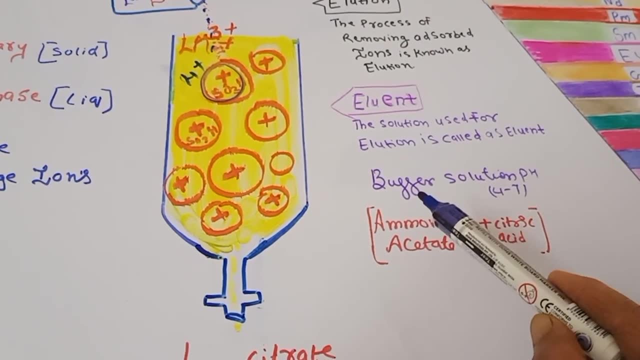 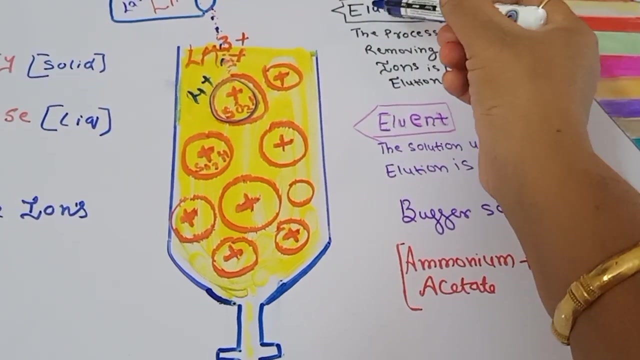 some eluting agents. so eluting agent is our buffer solution. what is elutant? so the solution used for the elution is known as the elutant. so here we are using the buffer solution, that is, a mixture of ammonium citrate and the citric acid. so when we will use our elutant means when we will do the 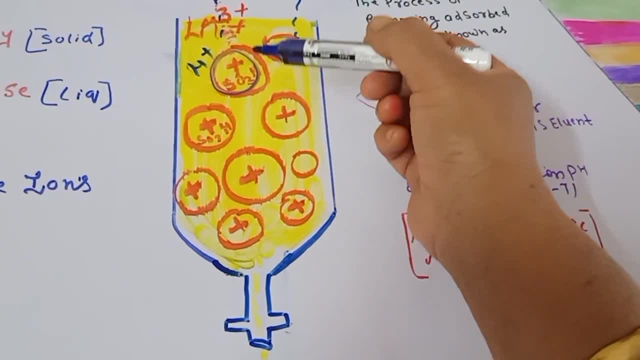 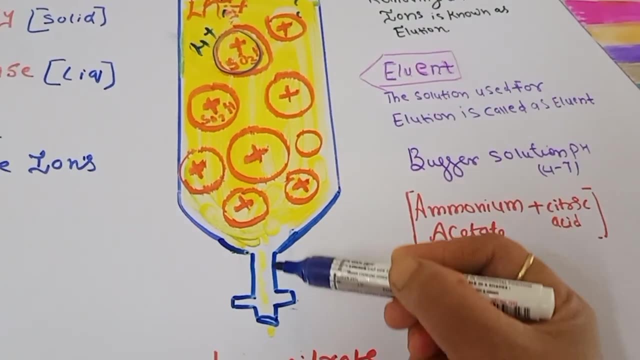 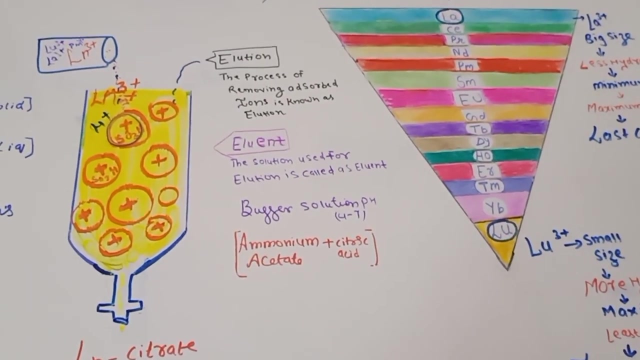 elution. so one by one, according to the which lanthanide attached with the resin firmly, means which is attached with the least firmly, will comes out first. Here you can see in the lanthanide series, our the size, as you all know that due to the lanthanide, 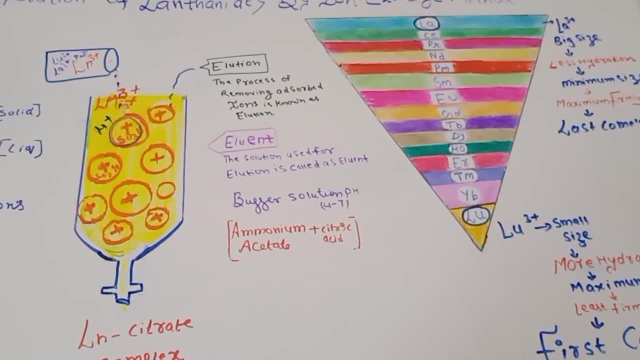 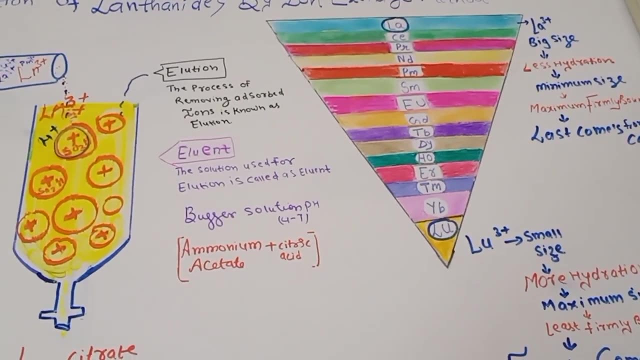 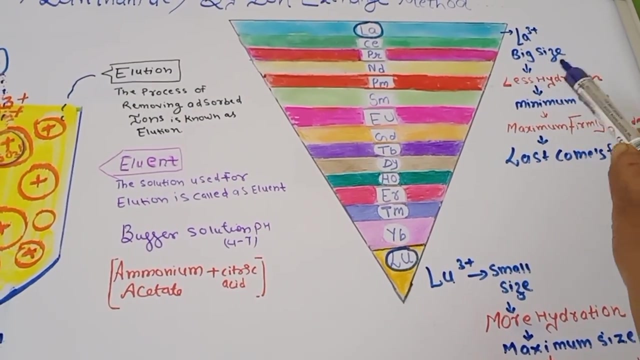 contraction. our lanthanum ion is the biggest in the size and lutetium is the smallest in the size. So what happens here when we talk about their? how they will behave with the resins. So what happens here? as the lanthanum ion is big in size, so it will be least hydrated means when they are. 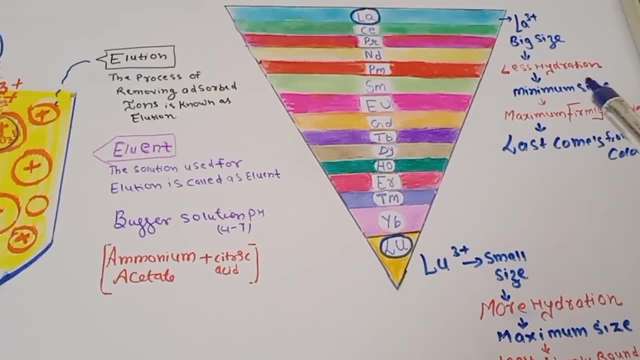 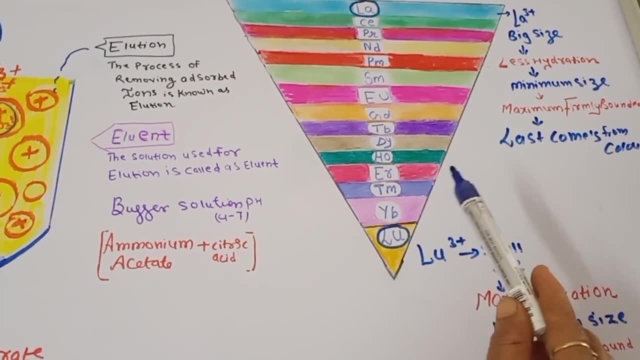 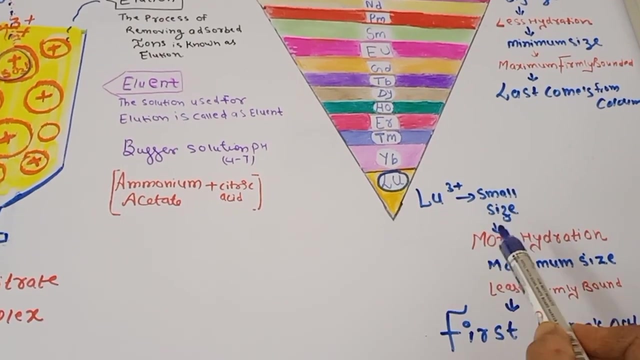 in the solution they will pass. their hydration will be minimum, so size becomes minimum and due to this it is maximum, firmly bounded with the resins. so it will come last in the column and as our lutetium. you can see, this is small in the size, so it will be more hydrated and it as the 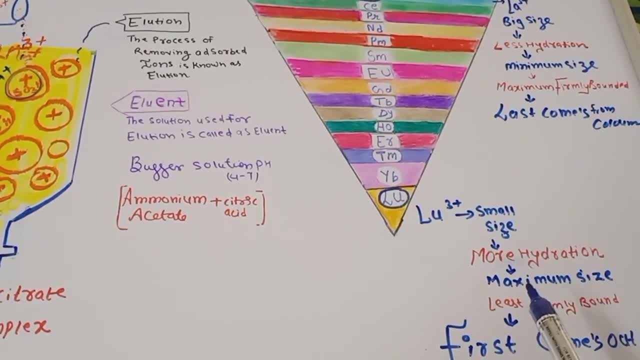 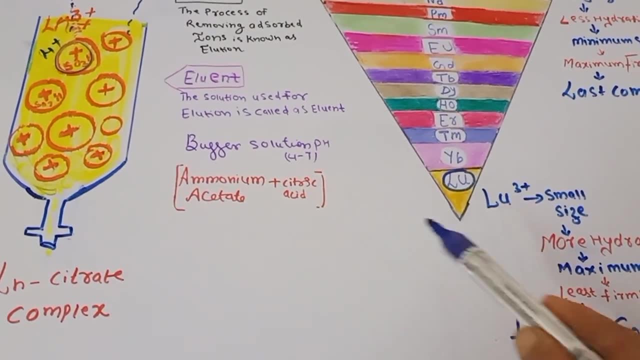 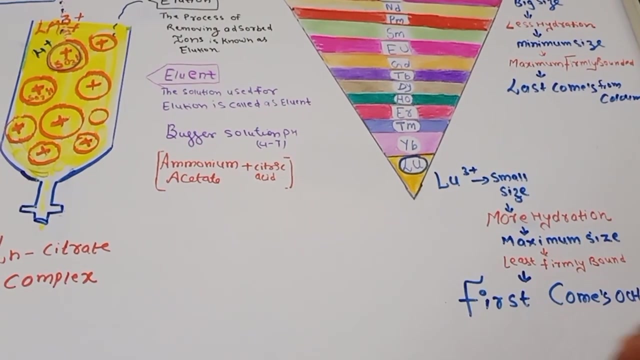 hydration of lutetium will be more, its size will be maximum and it is least firmly bounded means it is attached very easily with the resins. least firmly bounded means they are attached less firmly with the resin. so it will come first out of the our column. so, just so you can see this, what is the basics of? 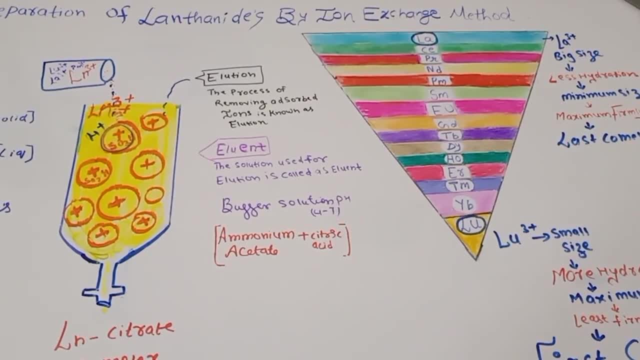 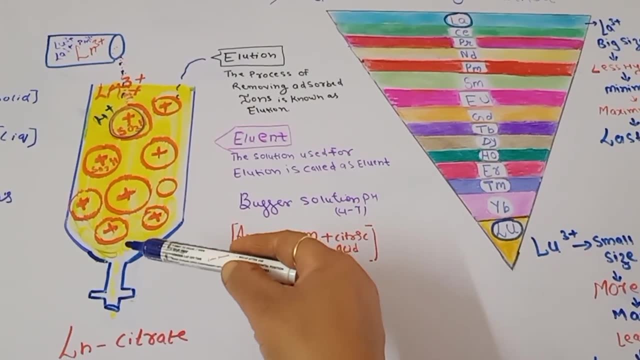 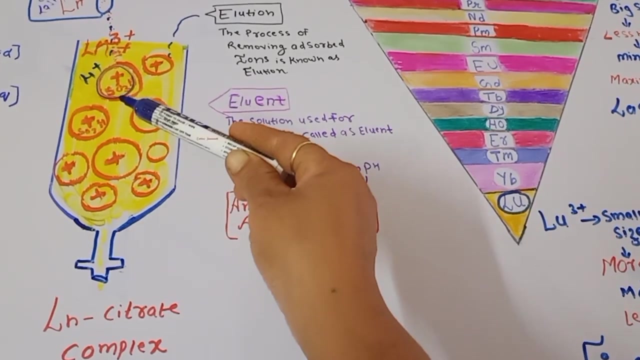 here what we have to do in the ion exchange method. we will take our solution or the mixture of the lanthanides and we will pass it through the bed of the resins stationary phase, and this ln3 plus will exchange with h plus and to remove this ions from this resin. 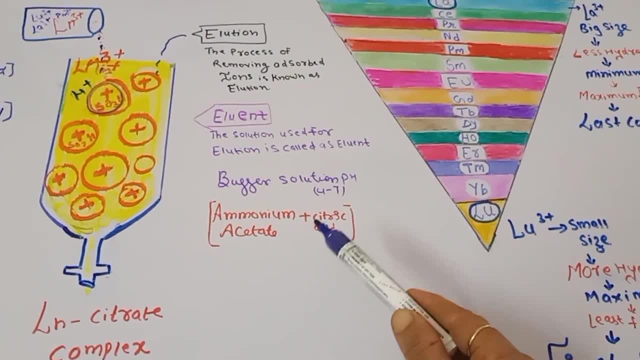 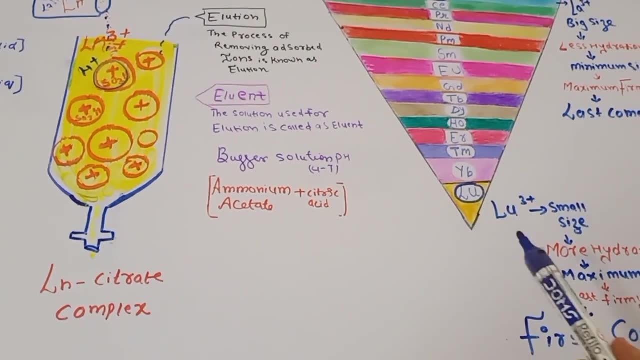 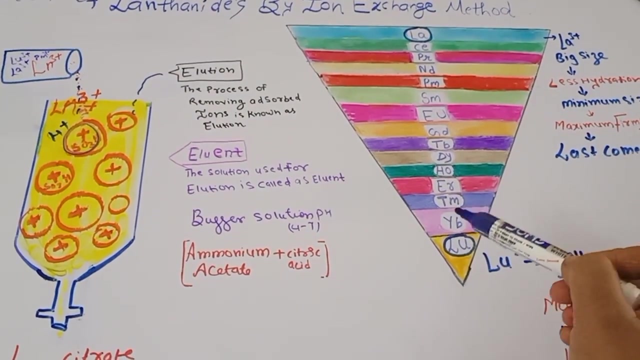 since what? we will use a buffer solution, that is our eluting agent. and when we will flow this buffer solution. so the ion which is attached least firmly, which is attached least firmly here, our lutetium. so you can see, here the tightly hold ion is our lanthanum. so it will come in the last and least. 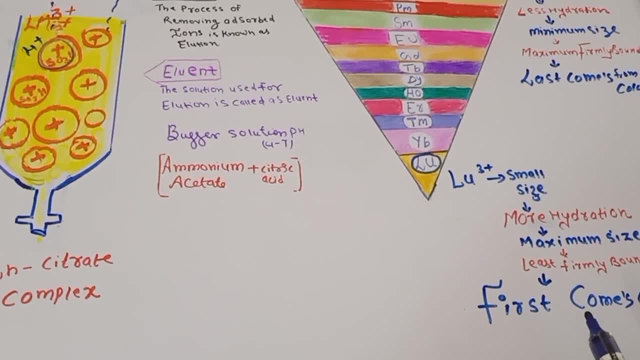 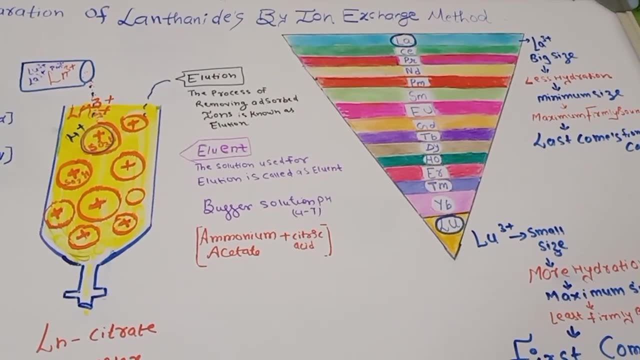 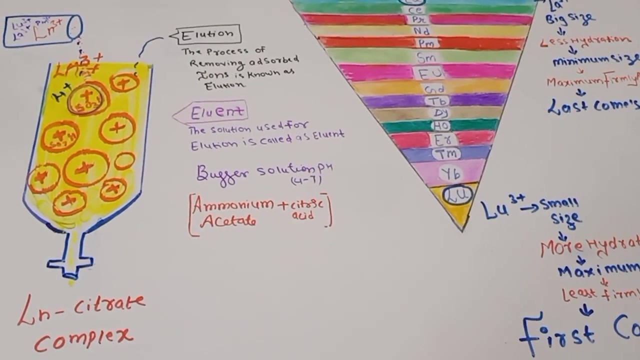 firmly bounded is our lutetium, so it will come our first, the first ion which will be separated in ion. third will be our lutetium, as the size is small, so it is the more hydrated and so it at least firmly bounded, so it will come our first out of the column, as is lanthanum citrate complex. so this 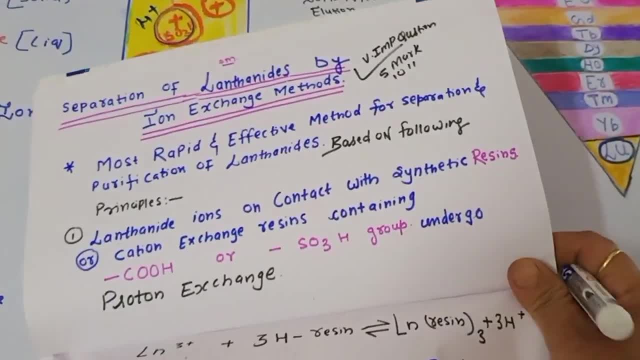 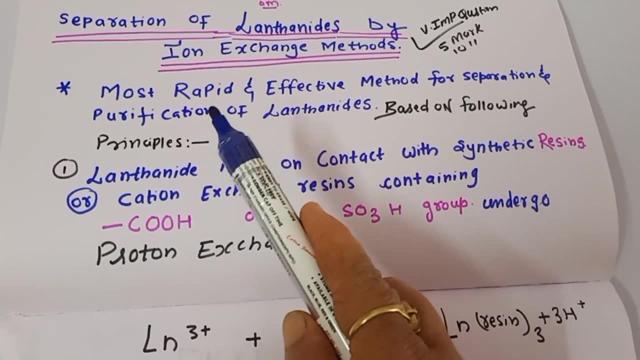 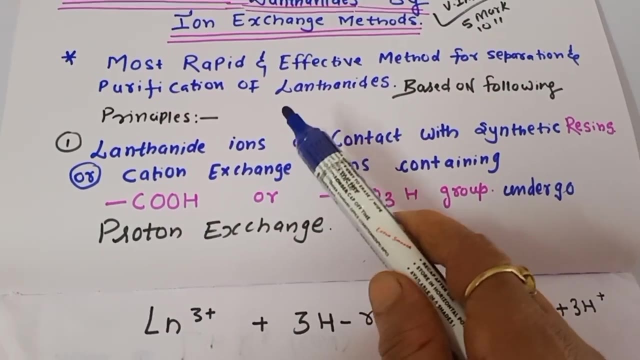 is for the, your means. just explanation. now you can write down the notes, so just i will read them fast. you can take the screenshot. most, uh, our ion exchange method. it is the most rapid and effective method for the separation and the purification of the lanthanides, which is based upon the following: 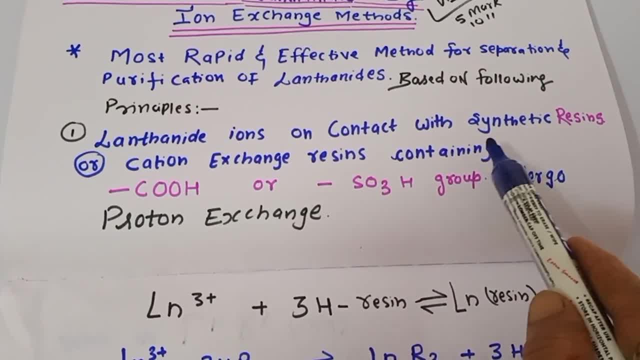 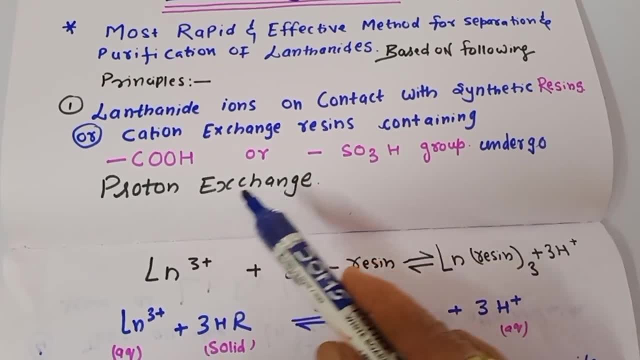 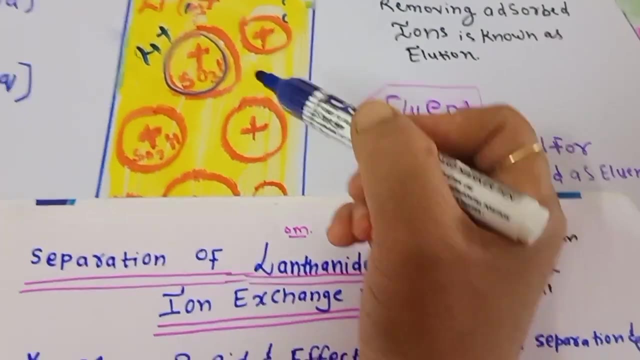 principles, the lanthanides, ions on contact with the synthetic resins or the cation exchange resins containing our carboxyly group or the sulfonic acid group undergo the proton exchange. as i explained you what they will do, they will undergo the proton exchange means so3h. h of this will be. 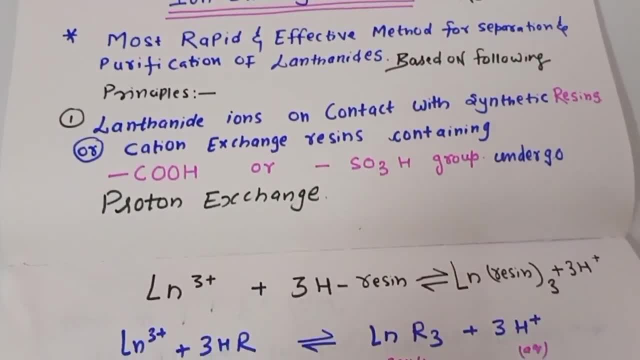 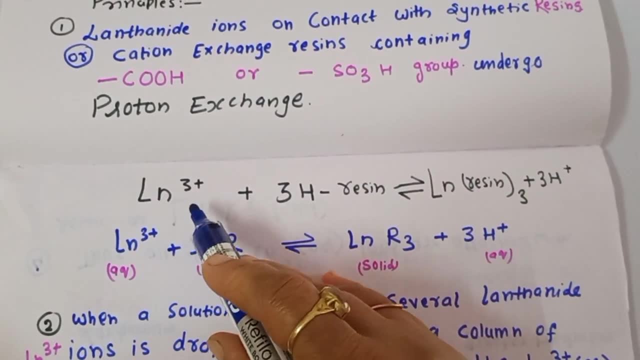 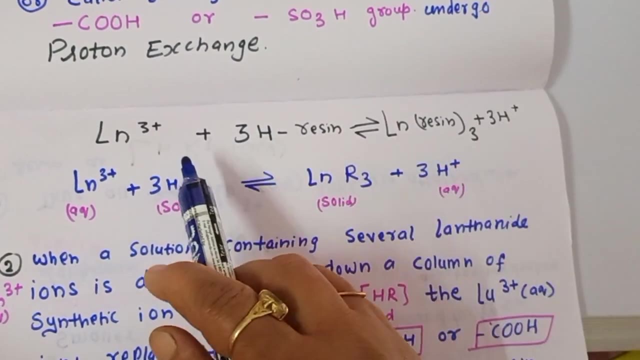 exchanged by our any lanthanide ion. then the next. just you can see the reactions, how they will be: isi possessions, the polyscarbon lieber которого. but the contact reasonocer protocol, i know our reaction rodents is not that important. so how do we change the psychology of our rosens? its 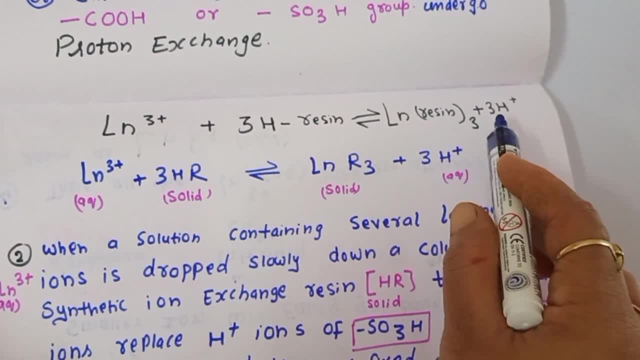 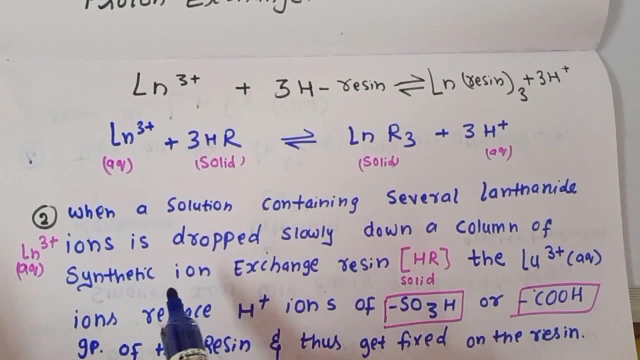 because our resins connect with a certain body Room in far greater than half the molecular onion distance. so if we add here to that myppersion of athletic, exist a resultation of two. all of my u- нев* coctail rbt provides such Carsonija techniques. so we give aás ready for green. 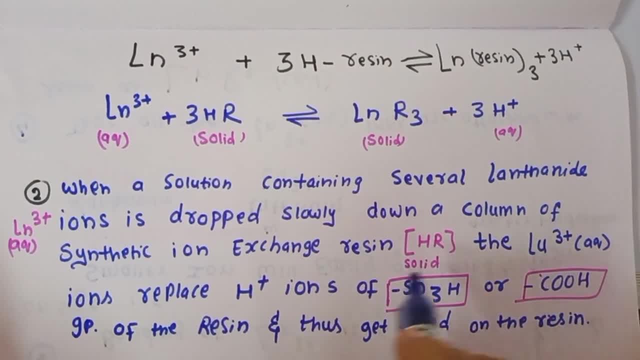 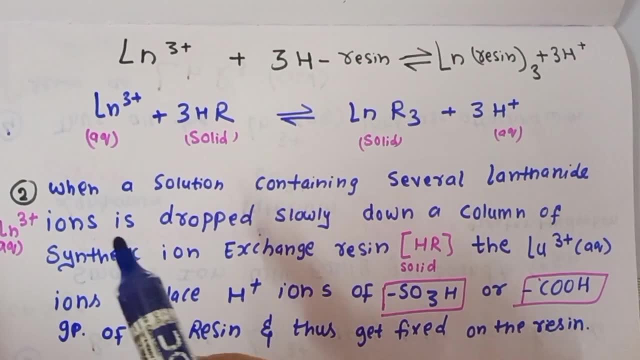 program percent. let's go further already. see now if we want costly H plus of the sulfonic acid group or the carboxylic acid group of the resin and thus gas fixed on the resin. so what is the main here? when we flow the solution of lanthanides, our H plus will be: 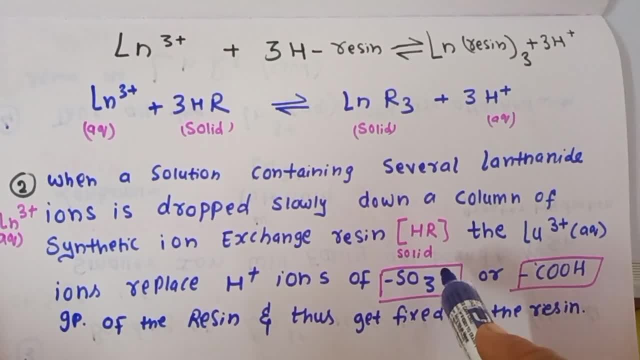 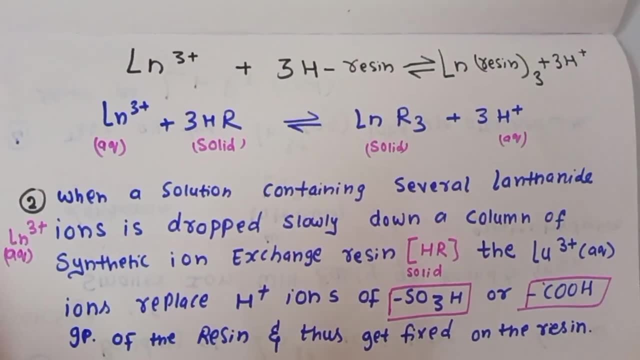 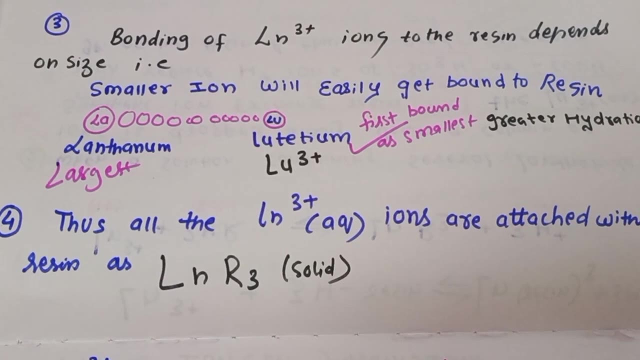 replaced by our lanthanide ions, suppose here if we will take Lu3 plus. so here what will become SO3 and Lu and they will get fixed with the resins. then bonding of the lanthanide ions to the resin depends upon their size, so which ion will be attached first, which ion will be? attached in the last. it depends upon their size, as I discussed that. lanthanum is biggest in size and lutetium is the is the smallest in the size, so a smaller ion will undergo more hydration. more hydration means they will be having the maximum size so easily. big size so it it will. 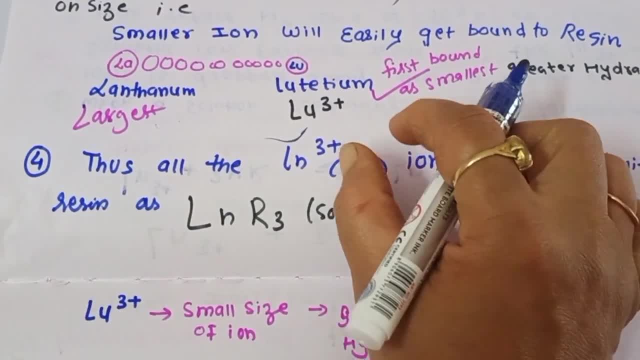 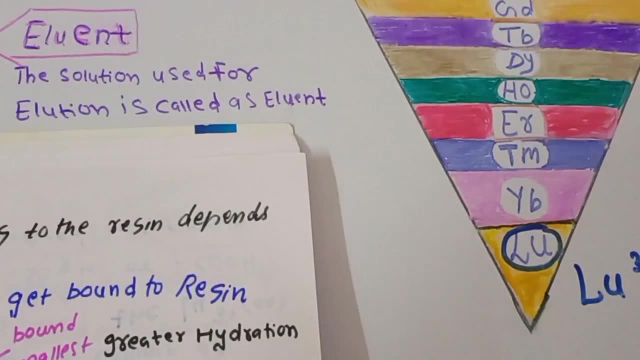 be easily bonded with the resin means slight bonding will happen between the resin, so as the light bonding means less bonding with the resin. it will be come out in the column, as you can see this diagram again, which will be come out first, our lutetium, as it is smallest in size and it will 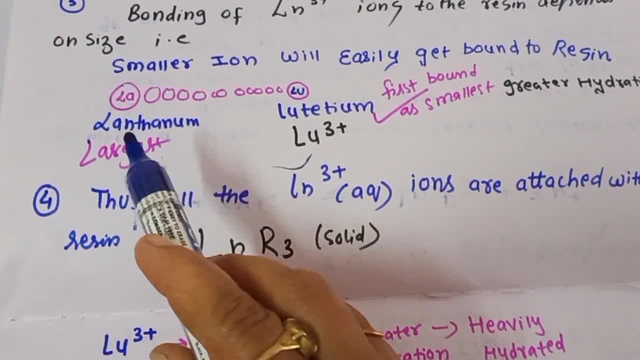 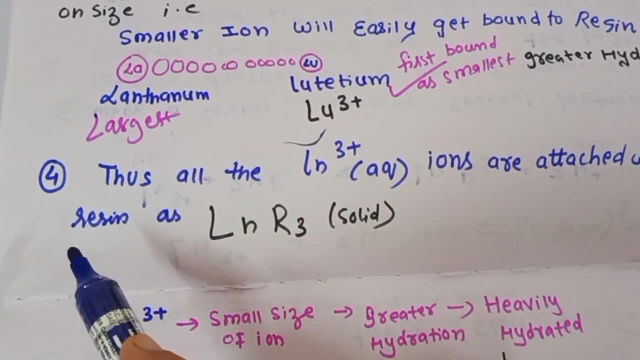 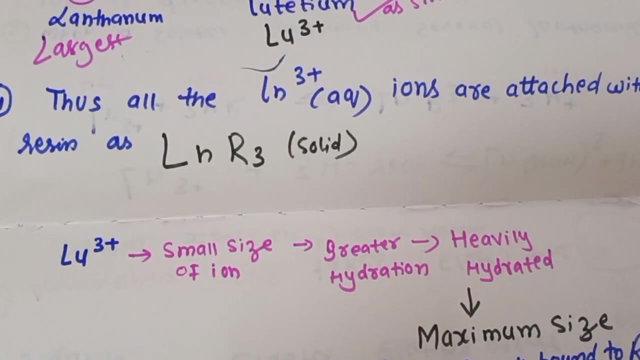 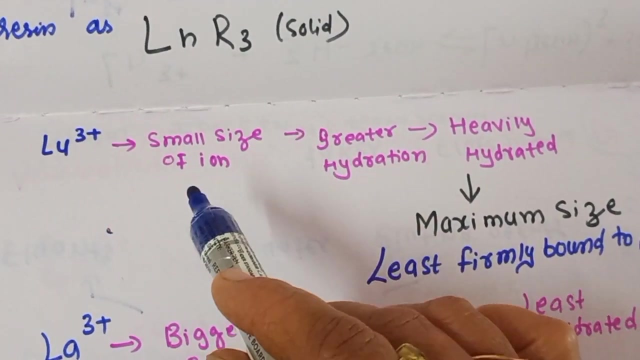 undergo the greater hydration. so when the lanthanum is bigger in size it will undergo the last. it will come last from the column. so thus all the lanthanide ions are attached with the resins as in the form lnr3. so just you can see that lutetium, as already discussed, lutetium is a small size. it will undergo. 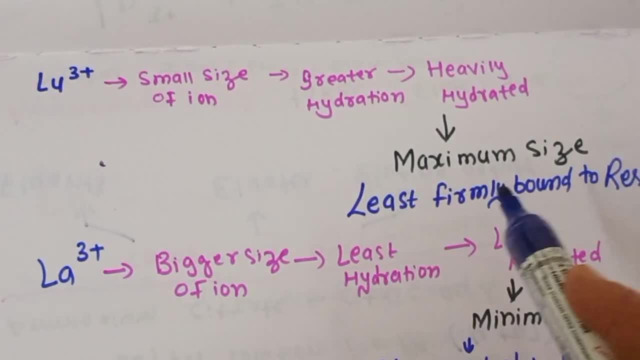 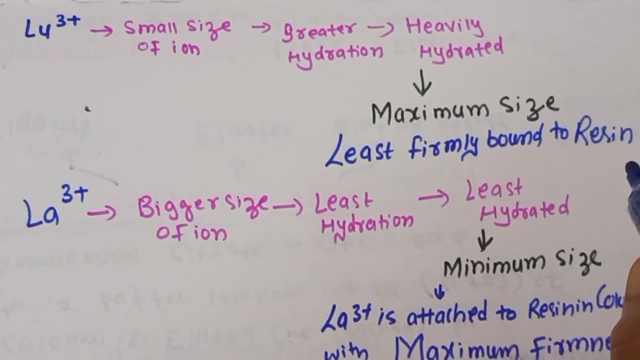 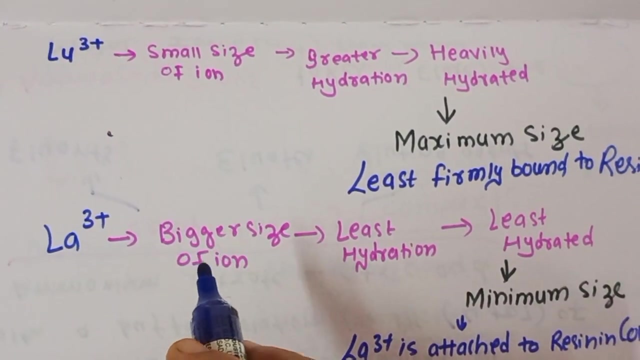 the greater hydration, so it will be heavily hydrated, and the hydration, more hydration, so size will be maximum and it will be least firmly bonded to the resin. so what happens here? similarly, the lanthanum 3 plus bigger size, it will be least hydrated. least hydrated means it will be bonded.